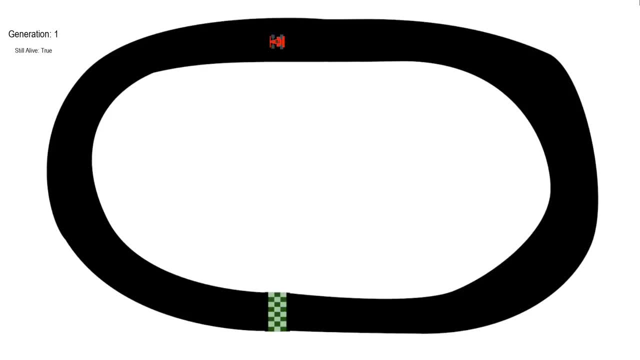 Machine learning is awesome, and one of the most exciting things that we can do with artificial intelligence on our own computers is running AI simulations. In this video, we're going to simulate the evolution of self-driving 2D cars in Python. For this we will use a technique called neuro. 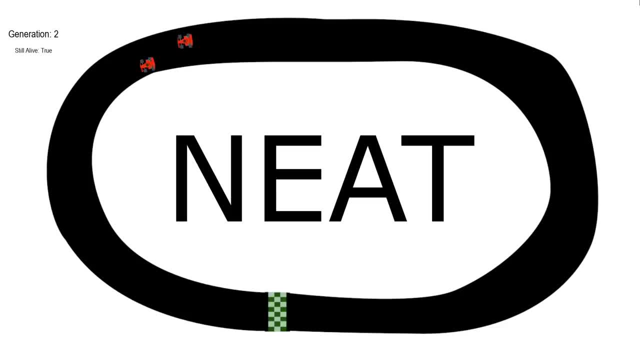 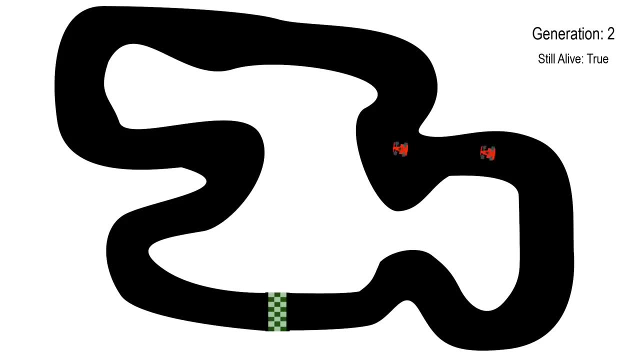 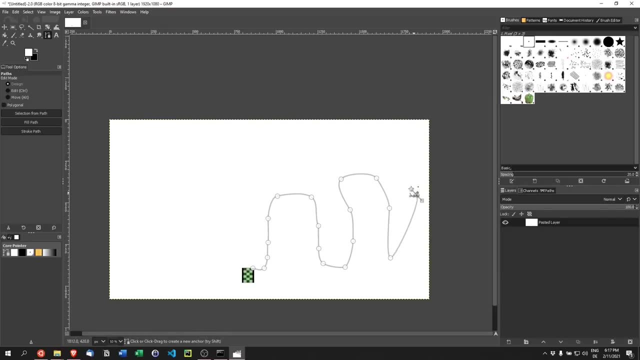 evolution of augmenting topologies- short NEAT. We will start with some very basic maps that are quite easy to learn and we're going to work our way up as we go on. The cool thing about this is that we can draw our maps with simple tools like paint or GIMP. We can try to design some smooth 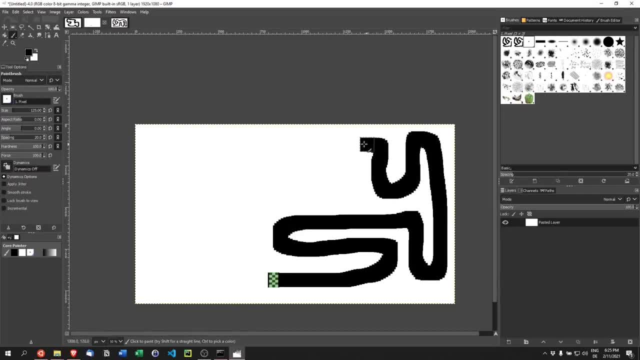 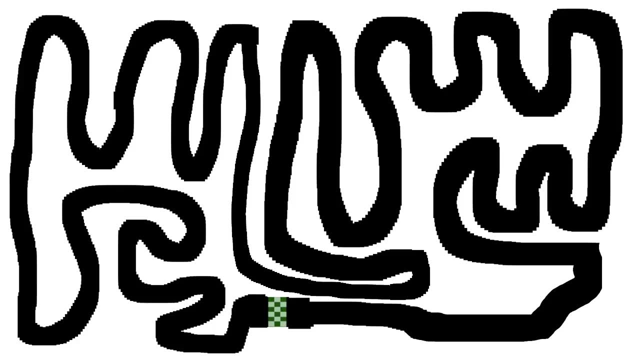 curves by using the path tool, or we can just pick a brush if we lack the patience for that. If we really want to challenge our models, we can also draw some crazy maps that look like this: Our cars have five sensors that look out for the borders. Those are the five input neurons of our 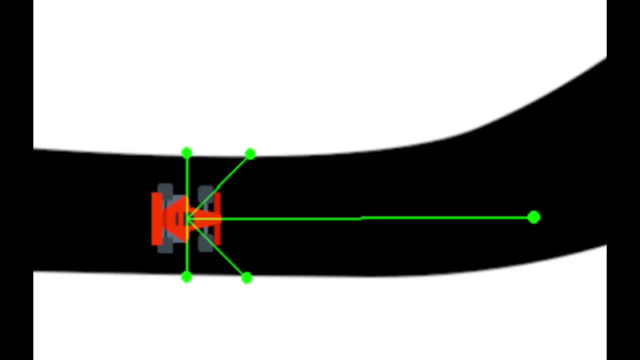 neural network. This is the only thing that our AI actually sees. Also, our model has four output neurons that represent the values of the捐s and the values of our AI. So our AI will be able to four actions it can take. Those are: steering to the left, steering to the right, increasing the. 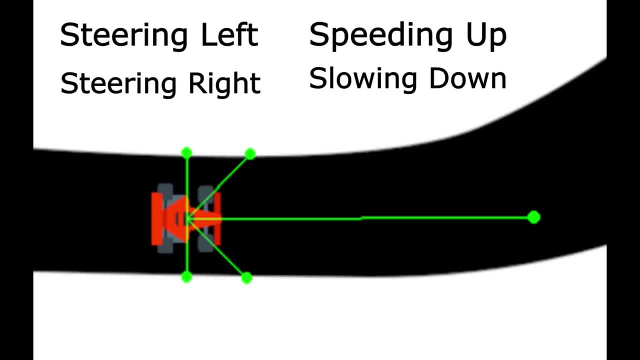 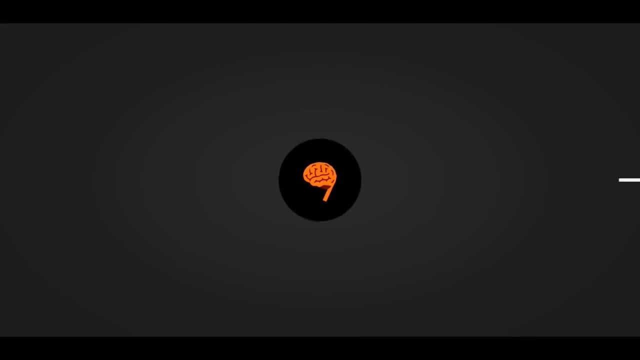 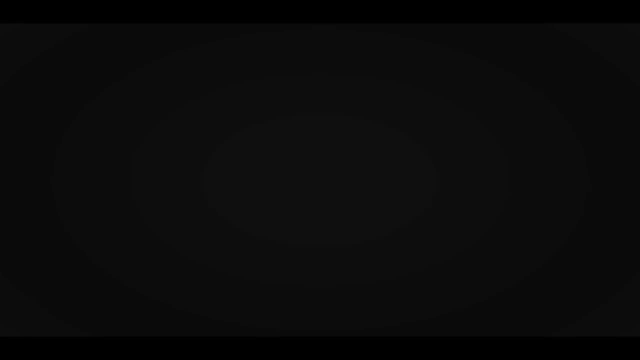 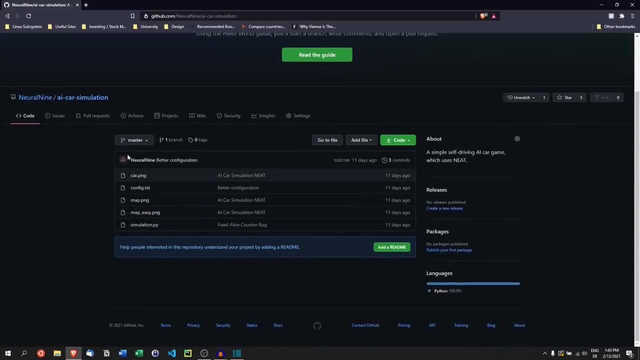 speed and decreasing the speed, considering a certain predefined minimum speed. So grab some popcorn, hit the like button and let's get right into it. First of all, I want to mention that the whole code is available on github and, heavily inspired by the youtuber Cheesy AI, I basically 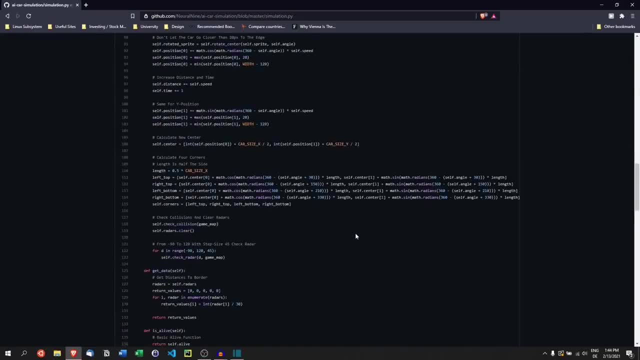 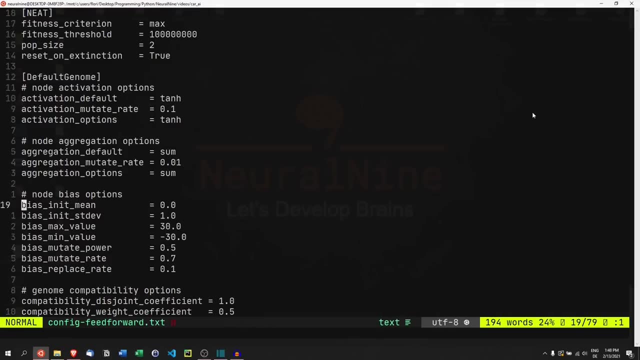 optimized and changed this code so that it suits this video's needs. The project consists of two major parts: the python file and the need config file. In the need config file we can specify all sorts of parameters which will influence things like reproduction mutations, the amount of 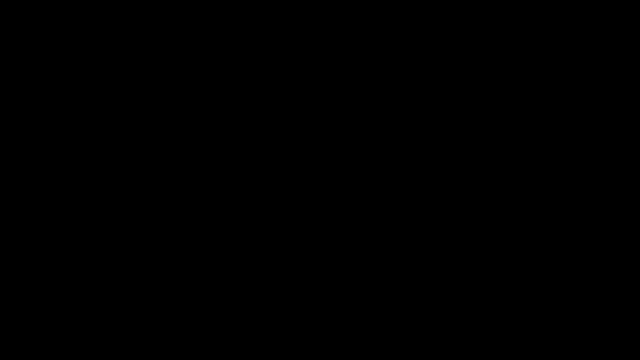 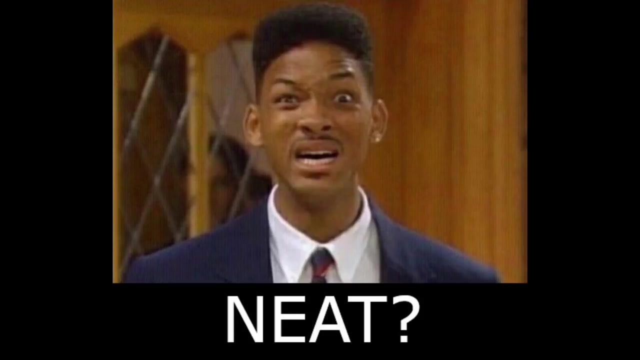 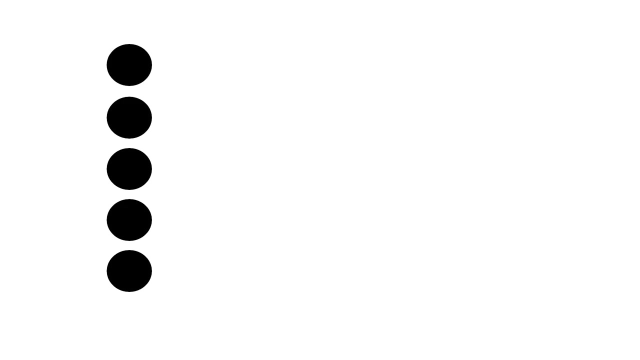 species, etc. For those of you who know nothing about need or reinforcement learning in general, I will quickly explain the basic idea of the whole code algorithm without boring you too much with any mathematical details, at least in this video. As I already said, our model is a neural network with five input neurons, the sensors and four. 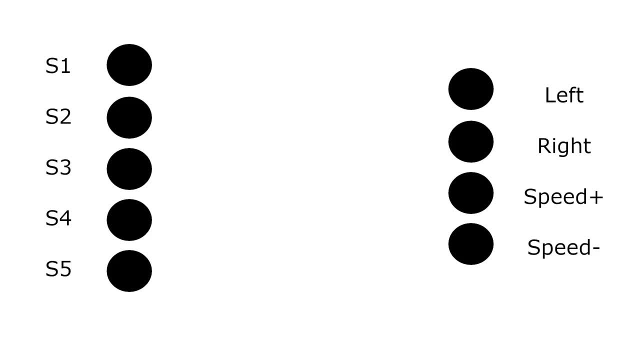 output neurons the actions it can take In between those. we can optionally have some hidden layers with additional neurons. Those layers increase the complexity and the sophistication of our model, but they also increase the training time and the likelihood of overfitting. All those neurons are 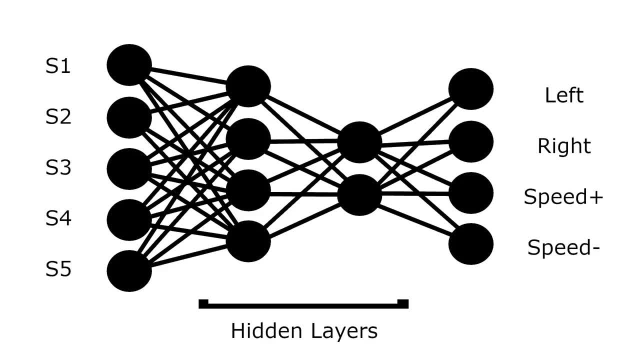 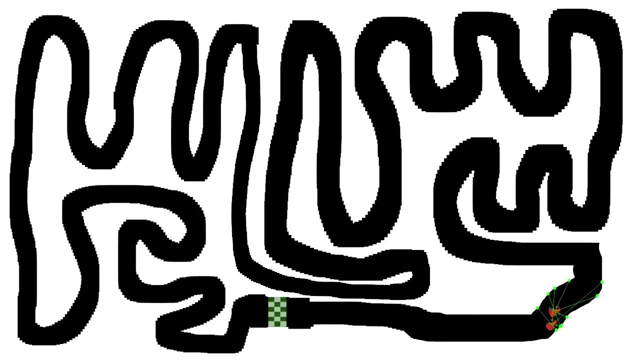 interconnected and those connections have certain weights Depending on the model's characteristics. the model will react in a certain way based on the inputs In the beginning. all those reactions will be totally random. there will be zero intelligence behind what our cars are doing. However, for each action our cars take, they will either receive: 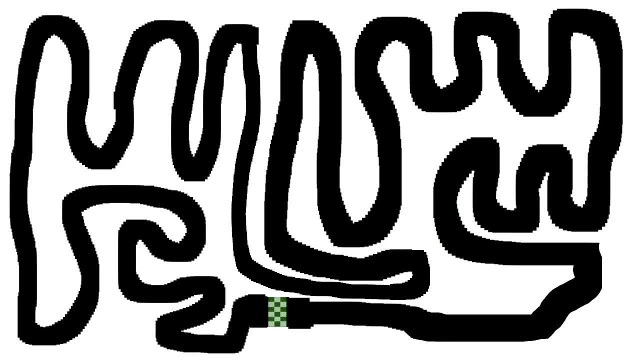 a reward or a penalty. To implement this, we use the so-called fitness metric. in our simple simulation, the fitness of a car increases depending on the distance it covers without crashing. After each generation, we then evolve our cars. The cars with the highest fitness value will be the ones which you can see here in the top right corner. 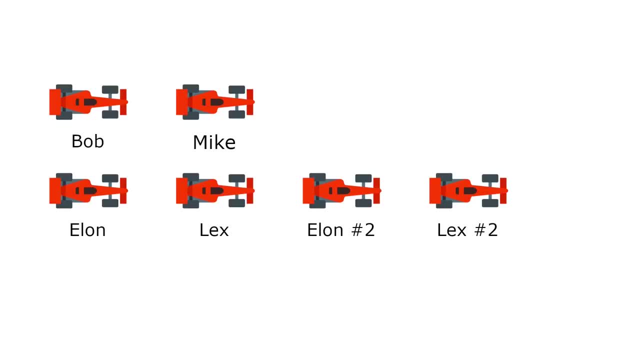 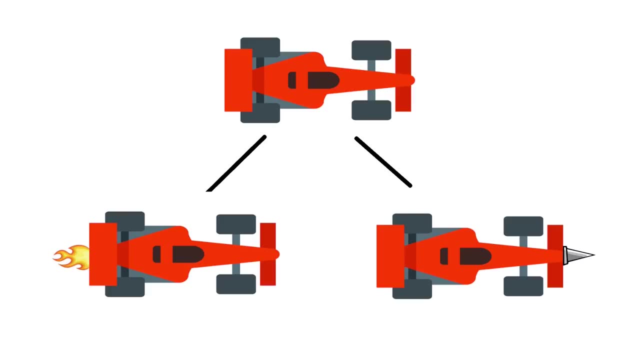 will probably survive and reproduce, whereas the cars that didn't perform so well will go extinct after a while. When a car reproduces, it will not just duplicate. the child car will be quite similar to its parent, but not the same. Therefore, it has a chance to become better Cars that are very 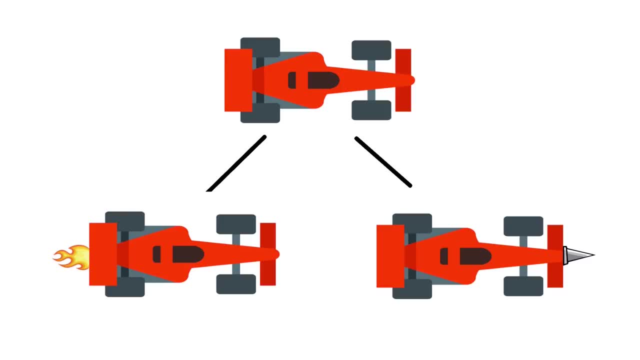 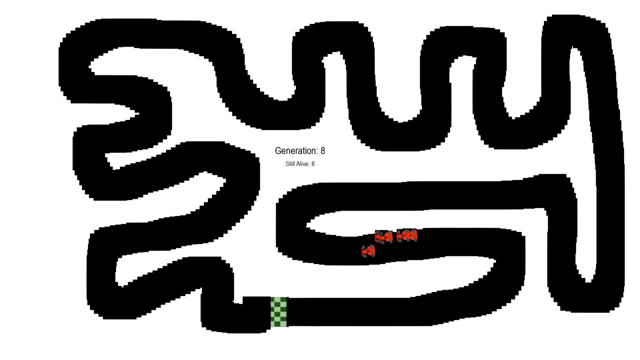 similar to each other form and own species. If a species doesn't see any improvements for a fixed number of generations, it goes extinct. Given all those principles, we can create an environment in which the best cars survive and reproduce, whereas the worst cars go extinct and the model is forced. 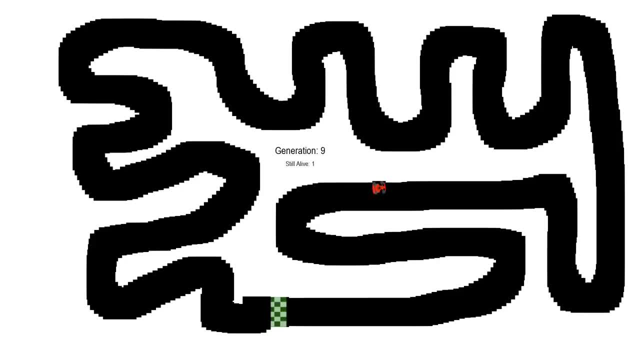 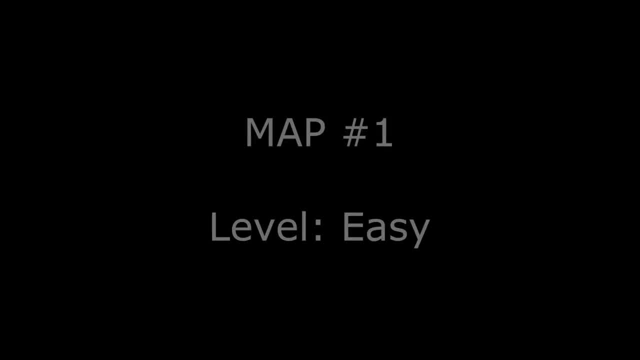 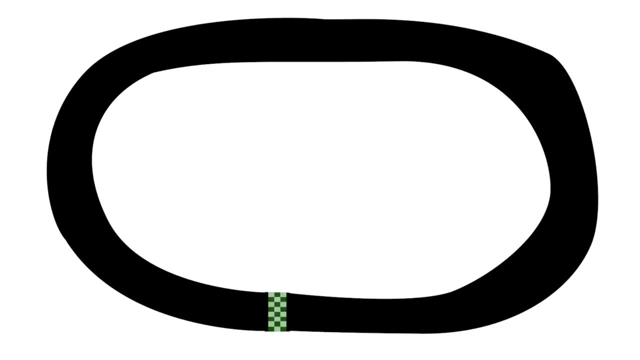 to experiment around. The basic principle is: what works will probably persist and be replicated. But I think that was enough theory. let's start driving For the first simulation. let us start with the most basic map possible, which is just a ring going full circle once, And the result is quite interesting, Since we have a population size. 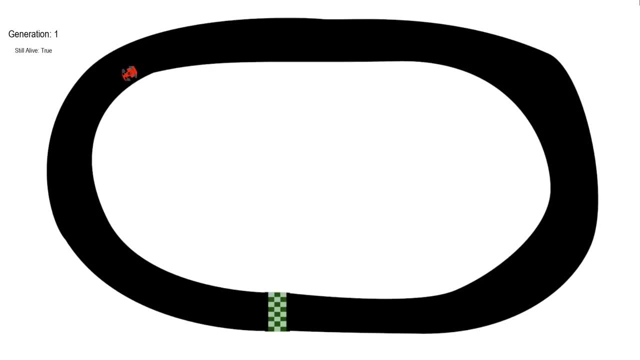 of 30 cars. they have to go around the circle to produce a set of models, And they need to. by mere chance, we already have a car that drives quite well in the first generation If we are interested in what's happening behind the scenes. 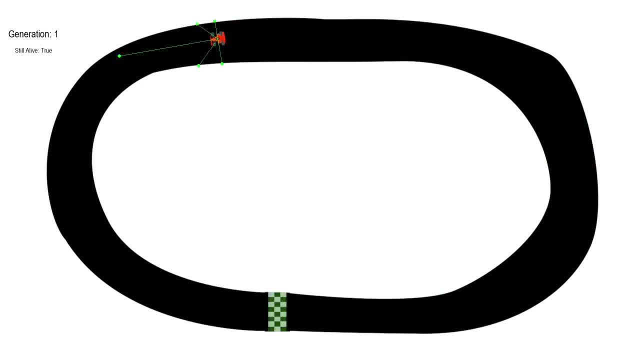 we can also show the radars to see what the car is seeing. The only thing that the car has to do is steer left in the right moment, and then it survives. In the next generation. we can already see that this car reproduced, and we now 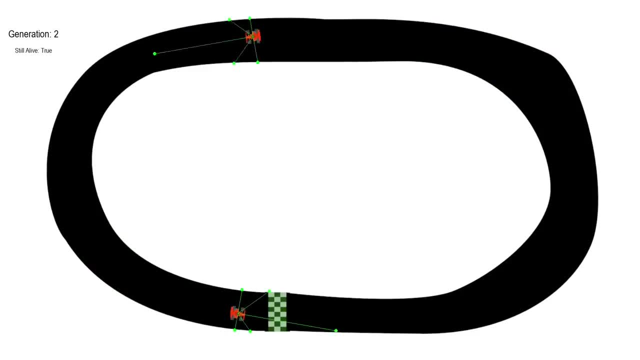 thus have two cars who are able to drive and not crash for 20 seconds. But not only that, one of the two cars is also way faster than the other one. This might have happened by mere chance as well. but remember: the fitness value increases harder the more distance a car covers in those 20 seconds. 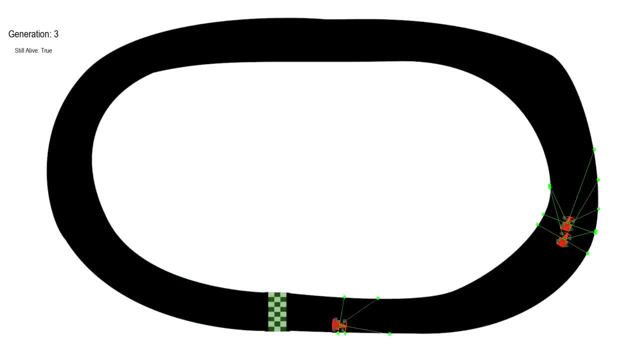 And our cars have the ability to accelerate. Therefore, if a car figures out that increasing the speed in the right moment leads to better results, we might see a new alpha species here, And in fact, in generation 4 we can already see four of those fast-driving cars. 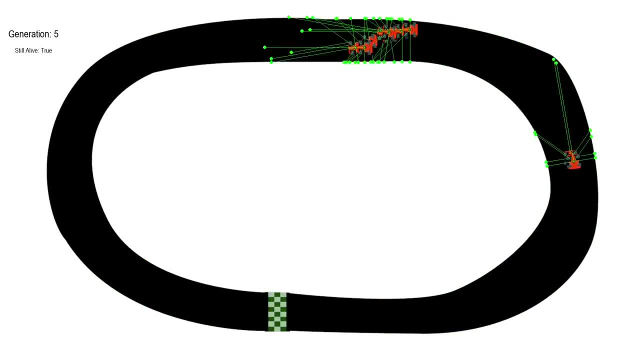 By generation 5, most of the cars are driving fast and you can even see one car making a very good attempt to drive faster than the other cars. And in fact, in generation 4 we can already see four of those fast-driving cars And in fact, in generation 4 we can already see four of those fast-driving cars. 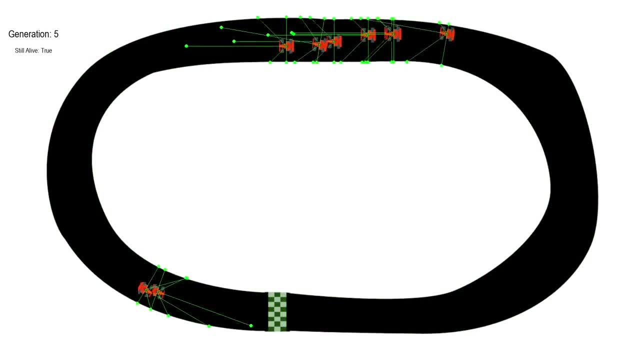 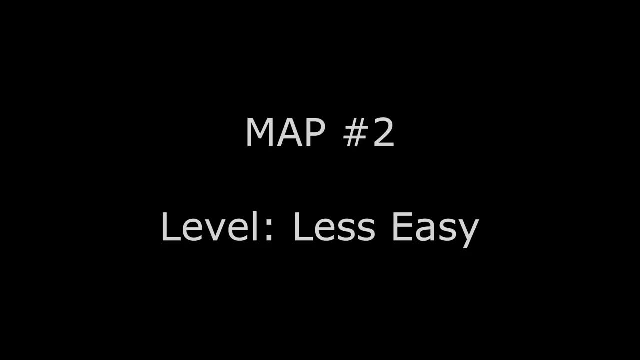 And in fact in generation 4 we can already see four of those fast-driving cars. But this map is pretty basic. Let us take a look at a map that has some more curves in it. Here, as you can see, every single car crashes right in the beginning of generation one. 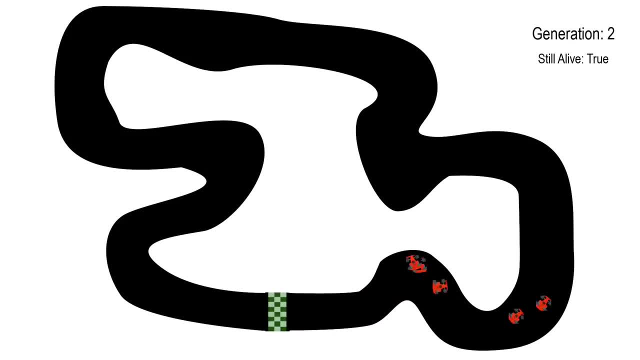 This seems to be a bit harder In generation two. we have some promising attempts, but still all the cars crash. And even though not a single car succeeds in the next couple of generations, we can clearly see that the quote-unquote best cars reproduce and we see more and more good attempts over time. 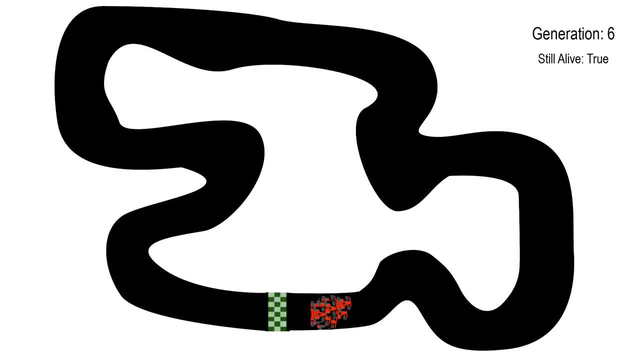 In generation seven. we can then, all of the sudden, finally see two cars succeeding at going full circle. One of them is going quite fast, whereas the other one tries to maneuver carefully through the racetrack. You can try and guess now which one will persist and reproduce over time. 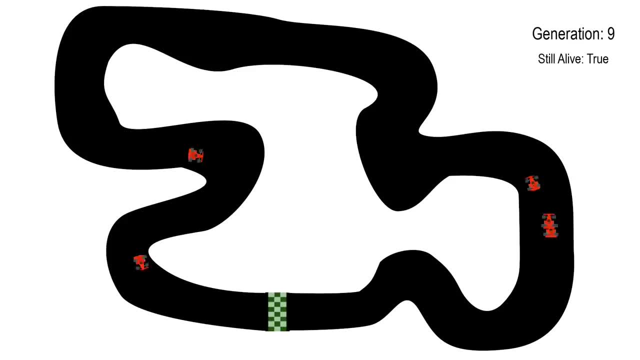 You can try and guess now which one will persist and reproduce over time. You can try and guess now which one will persist and reproduce over time, And maybe this comes as a surprise, but after 12 generations there are not too many differences between the two types of cars. 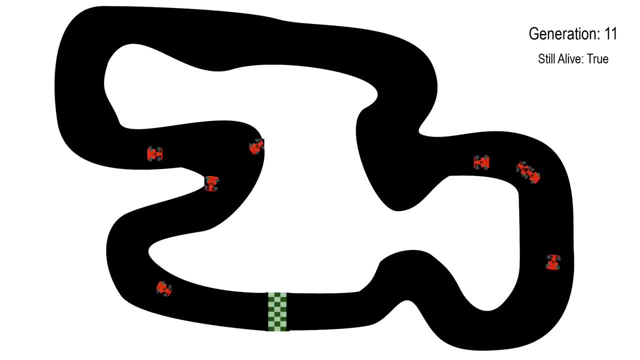 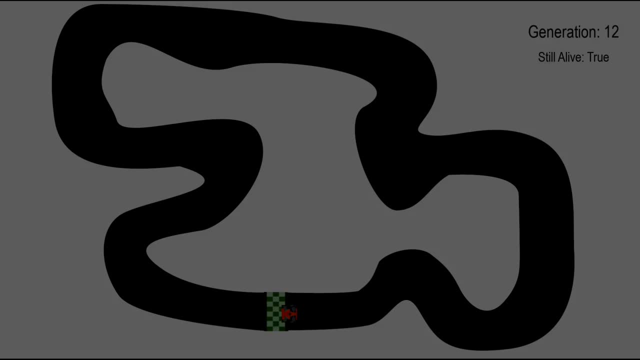 One explanation for this could be that, even though the fast cars have a better fitness value, the likelihood of a mutated version surviving at that speed is less likely than that of slower cars. This might definitely change after a couple of more generations, but let's go one level further, since this map is still quite easy. 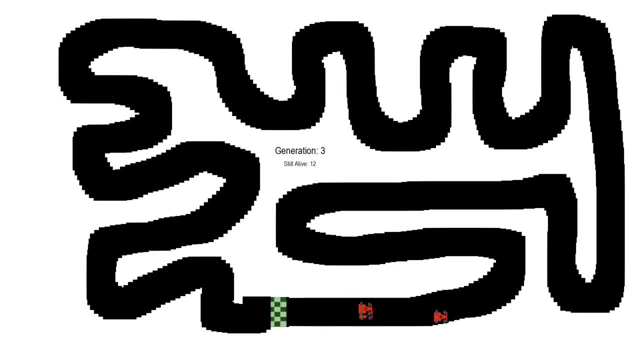 Now this map looks way more challenging, and it actually is. We don't see any meaningful improvements until generation eight, and even then it crashes soon after passing the starting curves And even though it tries to reproduce, even slight changes in the offspring lead to crashes. 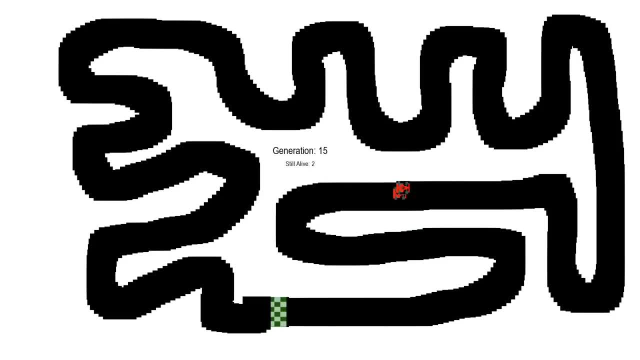 But then, in generation 15, we see a super child. This car does not only overcome the u-turn- its parent failed at multiple times- It even passes the full circle. It even passes the circuit in the first try- Very impressive. Since this is a longer track, I increased the time limit to 40 seconds. 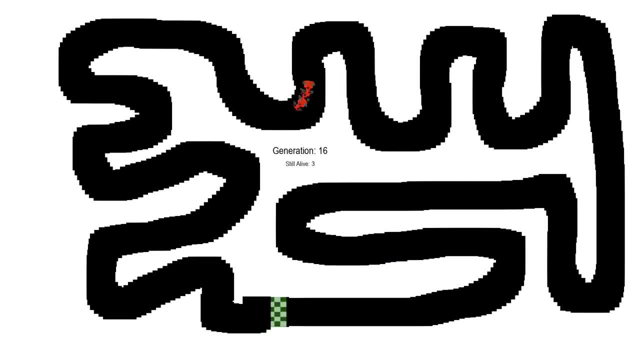 In the next generation we can already notice a reproduction. A second car managed to pass the full racetrack. However, doing that requires fine motorical skills, which is why many of the child cars fail after some curves. Then we notice something interesting: In generation 20 we have eight cars who managed to survive for 40 seconds. 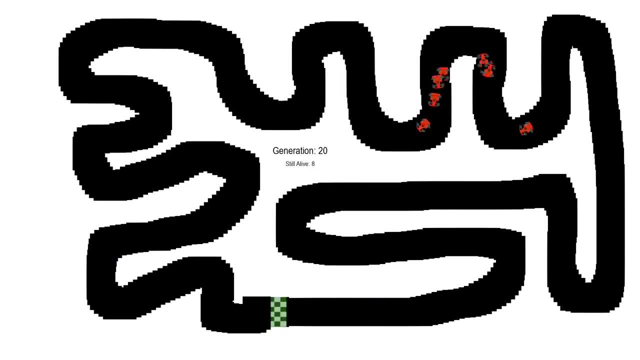 and cover a pretty good distance. However, in generation 21, that number has decreased to seven. Why is that? See the reason for that is a parameter called elitism. This parameter decides how many of the best cars will survive 100 percent. In our simulation, this number is set to two, which means that we guarantee that the best two cars will survive for sure. 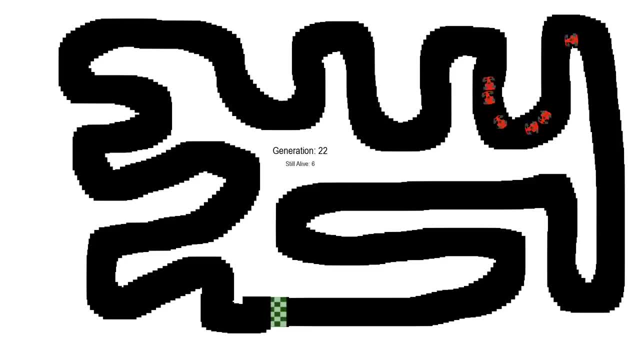 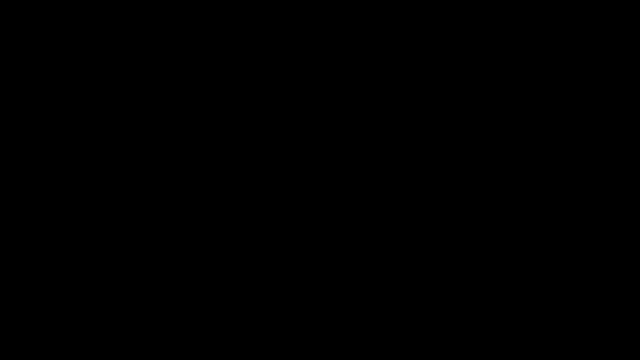 All of the other cars might die without reproducing, even if their results are quite good. Using those settings, we ensure that only the best of the best can survive and reproduce for sure. Since our model was able to beat every single map up until now, we will now try to challenge it way harder. 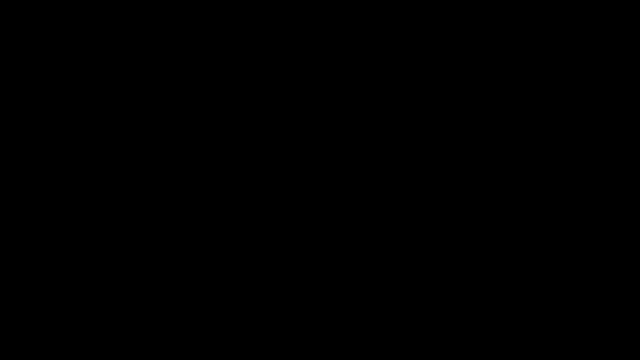 We will put our car onto a map that looks like something that a guy having a stroke would scribble onto a GIMP canvas in his last seconds. This thing is not only full of curves, it also has some pretty narrow passages that are going to be a huge challenge. 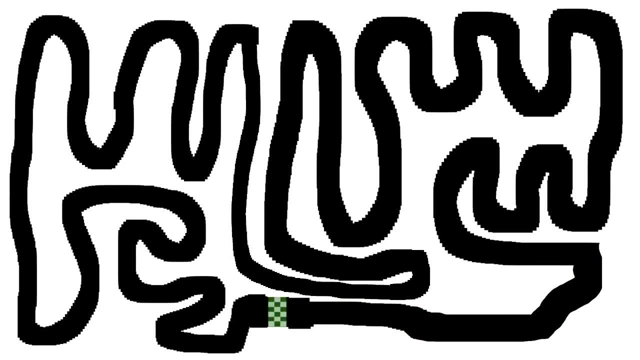 And, trust me, they were Naive as I was. I just started this simulation with the same parameters and settings as before And it failed miserably. I ran multiple simulations for hours and hours and the cars didn't seem to manage to pass through the whole track. 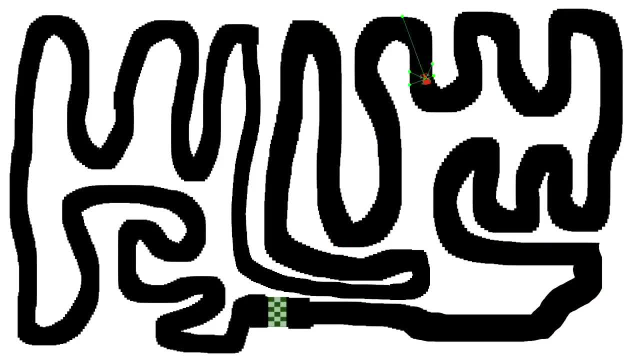 They made significant advancements and they even passed the narrow parts, but in the end they all crashed before reaching the finish line. So I thought: why not add some more complexity to the model? So I thought: why not add some more complexity to the model? So I thought: why not add some more complexity to the model? 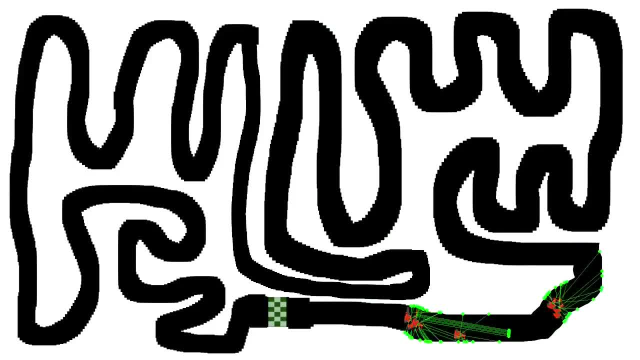 Up until now, we didn't use any hidden layers to increase the complexity of the model, So maybe this could help, But it didn't. I again spent multiple hours starting and restarting simulations. Not a single car managed to go through the finish line. 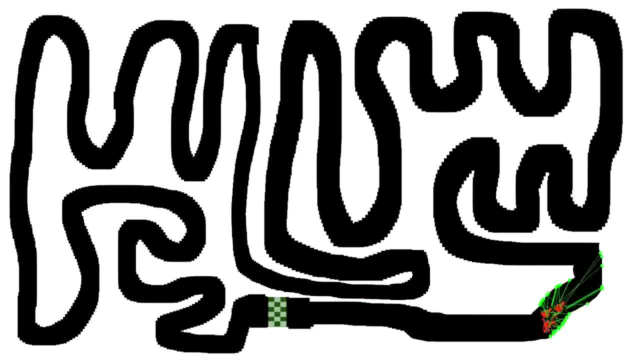 It actually performed worse with a hidden layer. It actually performed worse with a hidden layer. Now don't get me wrong. If we would run that simulation overnight, it would probably manage to cross the finish line sooner or later. But I wanted to find settings that get the job done fast. 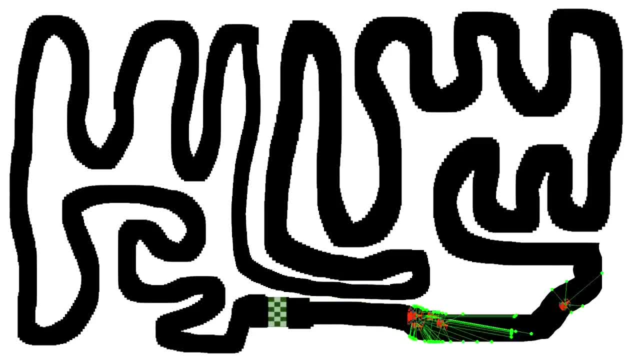 But I wanted to find settings that get the job done fast. So after experimenting around with the simulation, I found that it worked. So after experimenting around with the simulation, I found that it worked. So, after experimenting around with the simulation, I found that it worked. 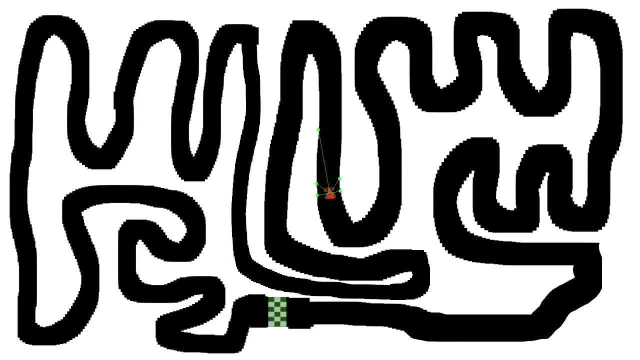 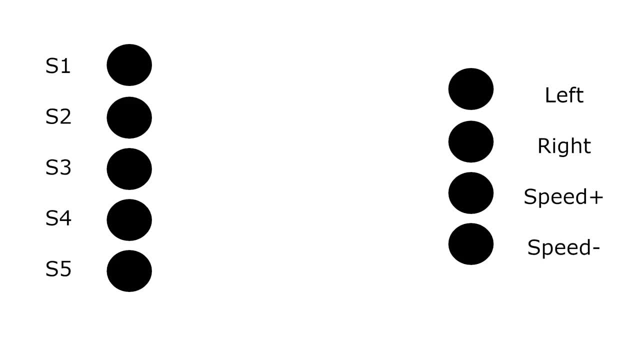 Maybe, instead of increasing the complexity of the neural network, I could simplify the choices it has. So what I did is I removed the hidden layer and also two of the output neurons. So what I did is I removed the hidden layer and also two of the output neurons. 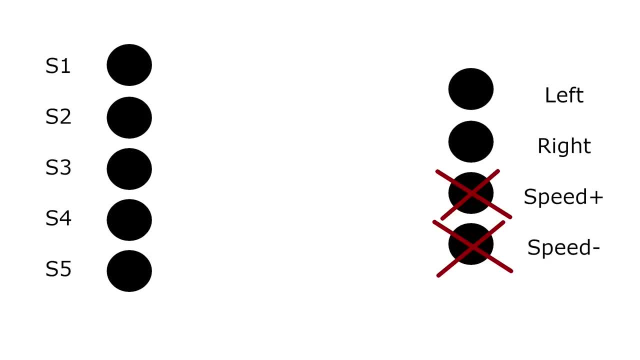 Those two output neurons were the ones which were responsible for increasing and decreasing the speed. Those two output neurons were the ones which were responsible for increasing and decreasing the speed. Those two output neurons were the ones which were responsible for increasing and decreasing the speed. 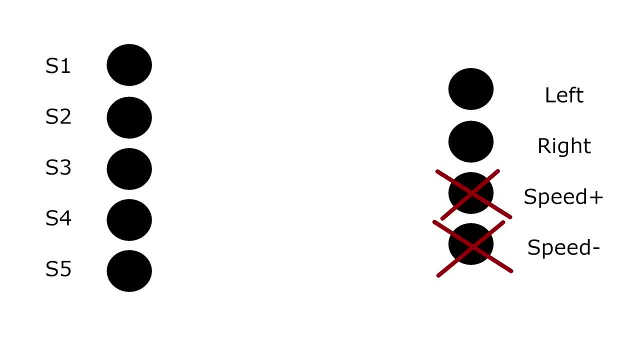 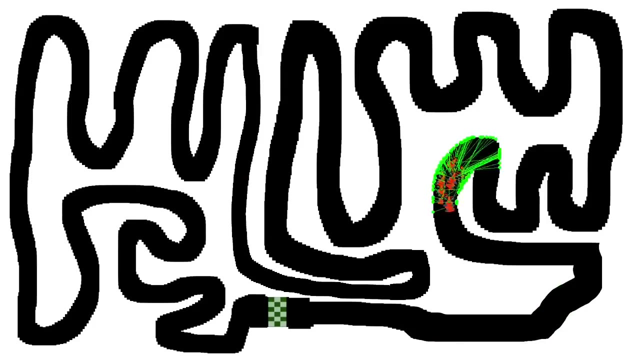 Instead of letting the neural network decide when to speed up or slow down, I decided to let the cars drive at a constant speed, To be precise at the former minimum speed, which was 8.. That way, the only thing that the model had to do was steering left and right. Notice that I didn't change any part of the 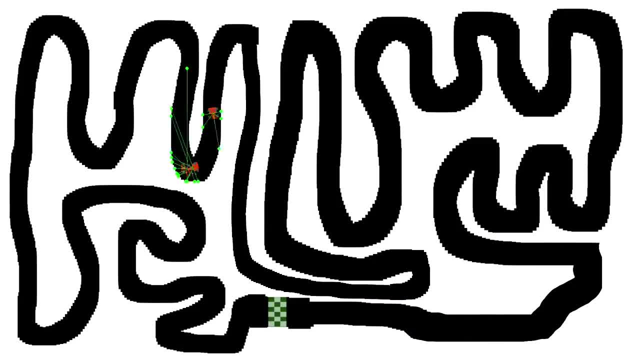 simulation, The car could have chosen that strategy on its own by just decreasing the speed down to the minimum and never increasing it again. So, technically speaking, we're not cheating. We just make a manual choice for the model so that it can focus on the steering, And even though it still took 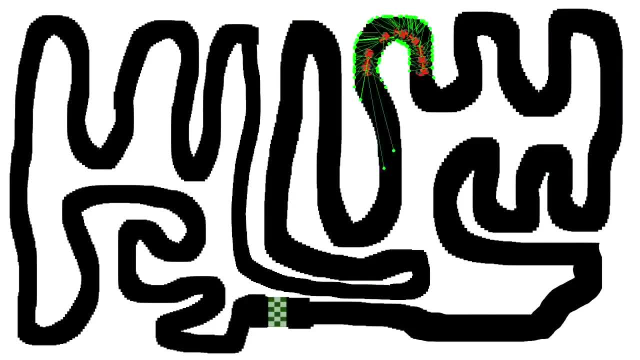 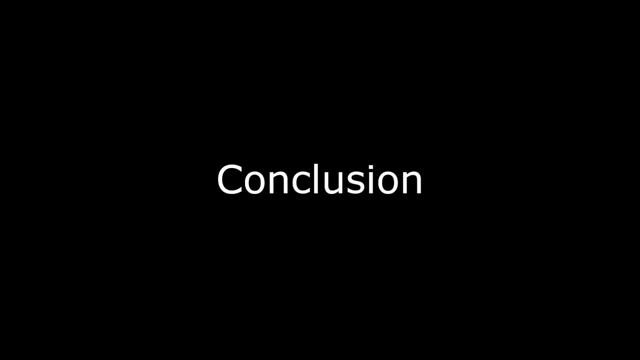 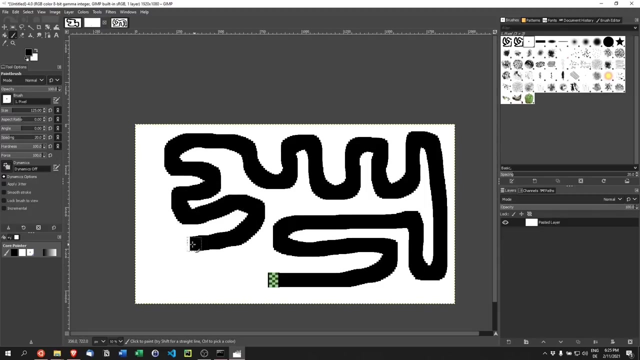 quite a long time, we actually managed to go through the finish line. using that approach, Simplicity wins. Now, of course, we could go on and on and create more ridiculous maps over time, but I'll leave that part to you. The code for this project, including the sprites, is: